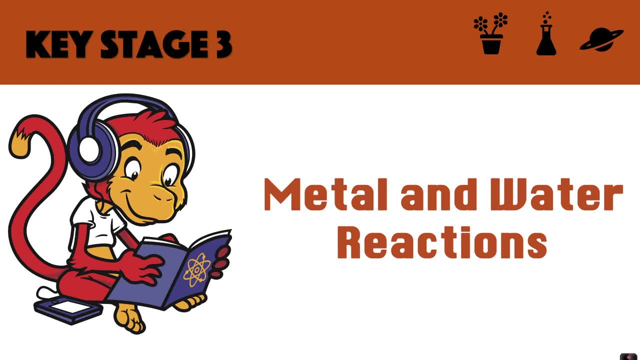 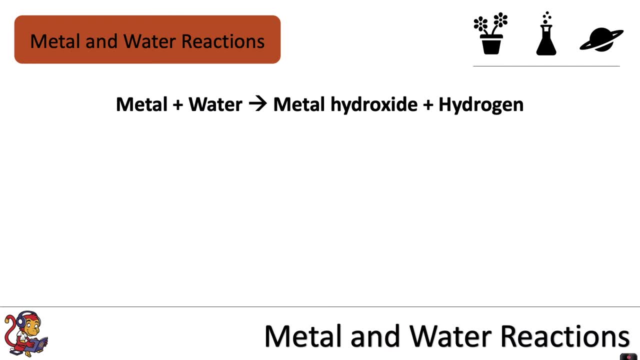 When a metal reacts with water, it produces a metal hydroxide plus hydrogen. So this is the general equation. Here is an example: When sodium reacts with water, it will produce sodium hydroxide plus hydrogen gas. And here is the symbol equation And we can use the 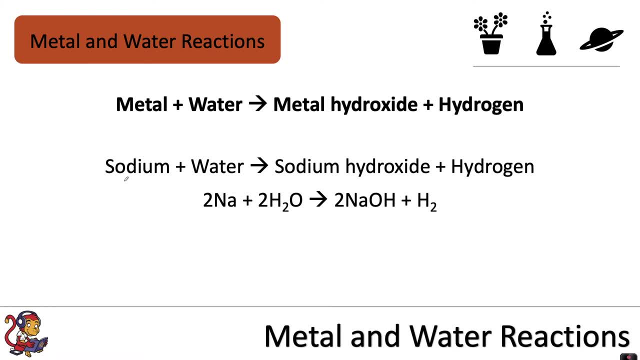 periodic table to help us get some of these symbols. So sodium is an element on the periodic table with the symbol capital N, lowercase. a Water has the formula H2O For sodium hydroxide. we take the sodium, which is from the metal, and the ending hydroxide is OH plus hydrogen. 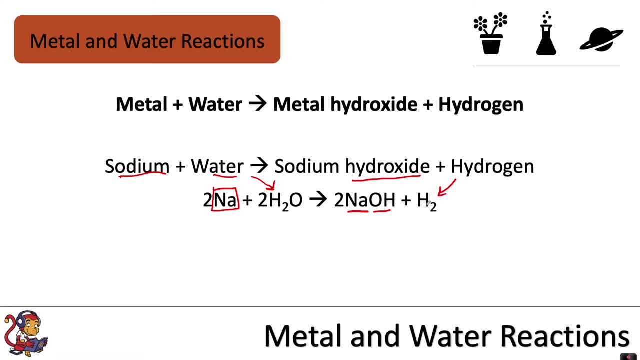 which always goes around as a pair. So we write that as H2.. And these numbers here are just used to balance the equation. So the symbol equation is: 2Na plus 2H2O would make 2NaOH plus H2.. In a second example, if 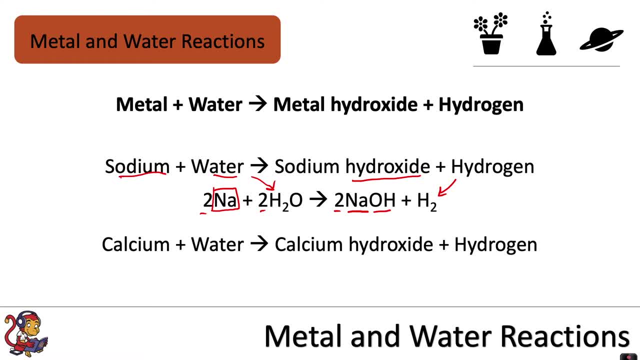 we reacted calcium with water, we would make calcium hydroxide plus hydrogen, And the symbol equation would be Ca plus 2H2O, would make CaOH2 plus H2O, So we write that as H2.. And these numbers here are just used to balance the equation. So the symbol equation is: 2Na plus 2H2O would make CaOH2 plus H2.. In a second example, if we reacted calcium with water, we would make CaOH2 plus H2.. And these numbers here are just used to balance the equation. And the symbol equation is: 2Na plus 2H2O would make 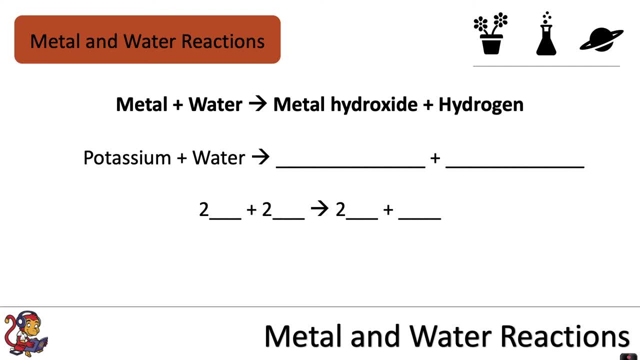 CaOH2 plus H2.. And these numbers here are just used to balance the equation. So here is one for you to try and complete And for the symbol equation, you can use the periodic table to help you. You might want to pause the video now whilst you have a go. 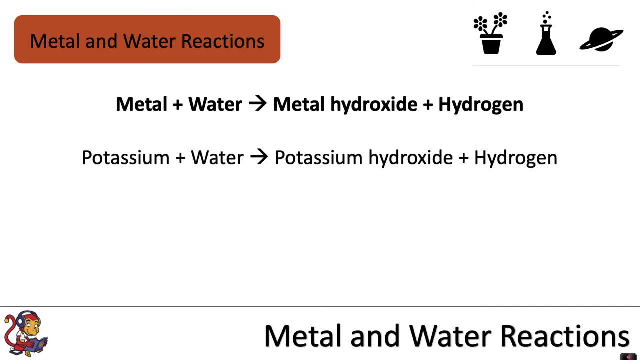 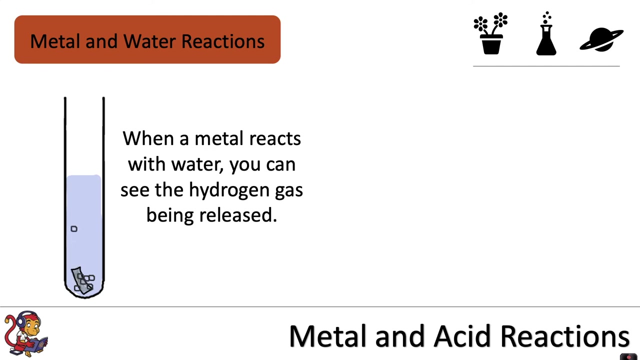 at this. Very well done. if you wrote that, potassium plus water would make potassium hydroxide plus hydrogen, And the symbol equation would be: 2K plus 2H2O would make 2KOH plus H2.. So when we react a metal with water, you can see the hydrogen gas being released.